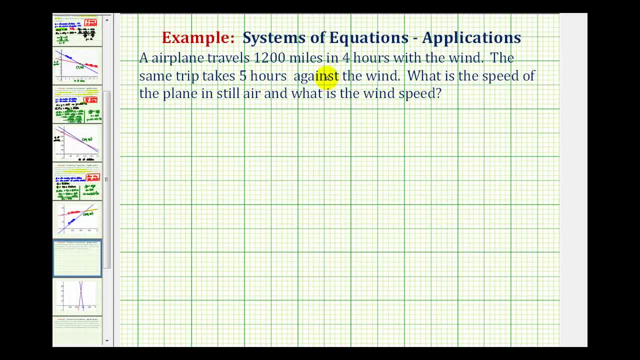 An airplane travels 1,200 miles in four hours with the wind, The same trip takes five hours against the wind. What is the speed of the plane in still air and what is the speed of the wind? So to solve this problem, we're going to set up a system of equations and then solve the system. 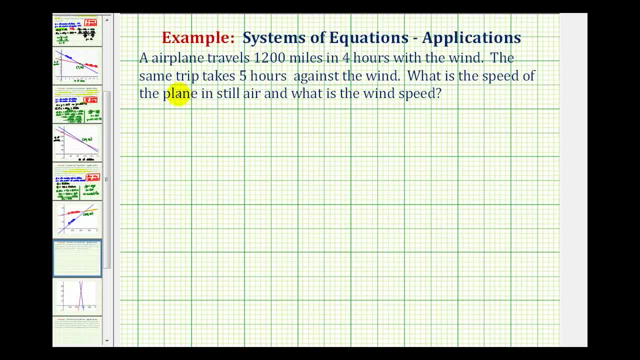 But this is also based upon the formula distance equals rate, times time, And our goal is to determine the speed of the plane in still air and also the speed of the wind. So let's let x equal the speed of the plane in still air. 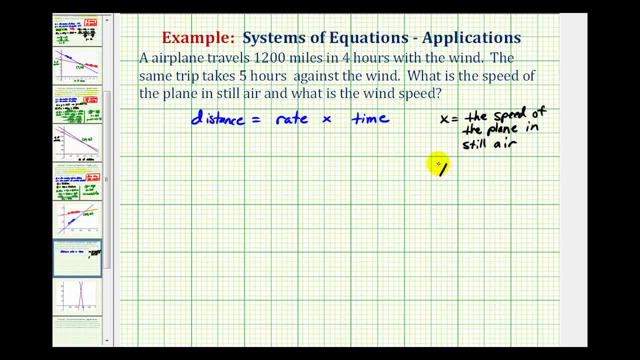 And we'll let y equal the speed of the wind. So we'll have an equation for when the plane is traveling with the wind And we'll have an equation when the plane is traveling against the wind. We'll notice, in both cases the distance will be 1,200 miles. 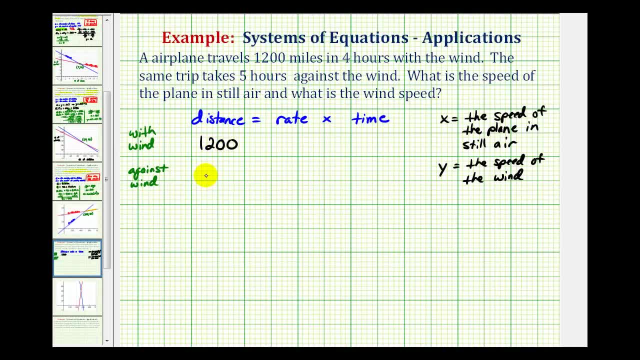 So we can put 1,200 here and here. Next, the plane makes the trip in four hours with the wind. So the rate when traveling with the wind is going to be the speed of the plane in still air plus the speed of the wind. 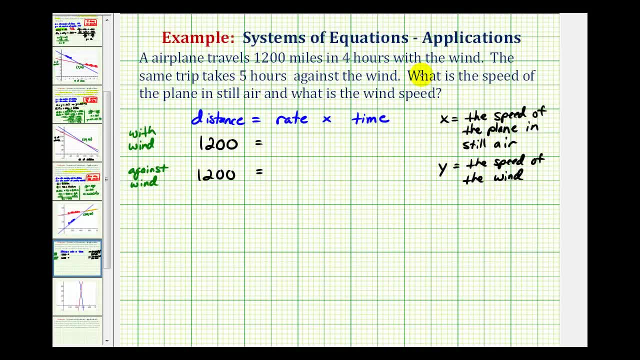 When the plane is traveling with the wind, it's making the plane travel faster, So the rate is going to be x plus y and the time is four hours, And then, when the plane travels against the wind, the same trip takes five hours. 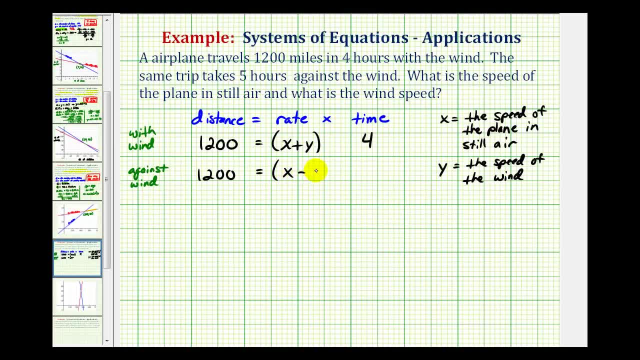 So the rate would be the rate of the plane in still air, minus the speed of the wind, because when the plane is traveling against the wind it's slowing the plane down. So this trip takes five hours. So here are the two equations for our system of equations. 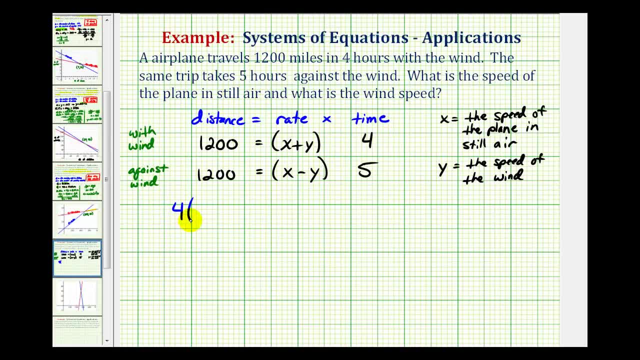 Let's go ahead and change the order of these. We'll write the first equation as four times the quantity x plus y equals 1,200.. We'll write the second equation as five times the quantity x minus y is equal to 1,200. 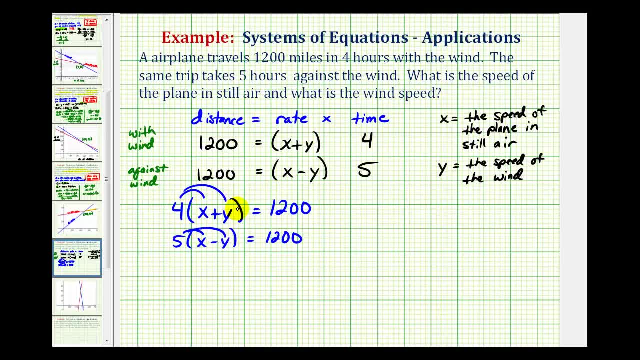 So now we'll go ahead and distribute. So that's going to give us 4x plus 4y equals 1,200.. And the second equation is going to be: 5x minus 5y is equal to 1,200.. 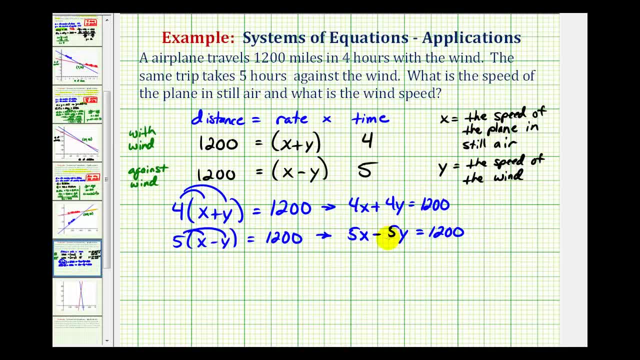 So to solve this system, we're going to need to write the following equation: So to solve this system of equations algebraically, we can either use the substitution method or elimination method. To use the elimination method, we want to add these two equations together. 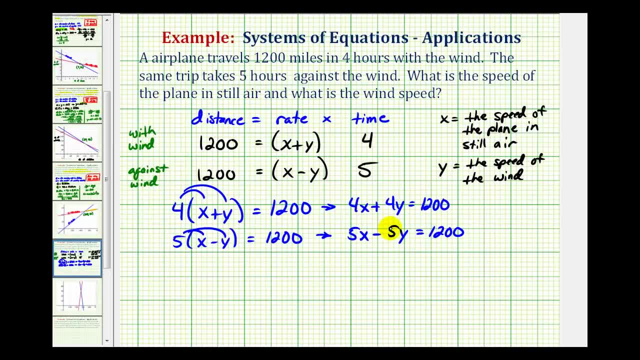 so that either the x terms or y terms have a sum of zero. To do that, they have to be opposites And we are going to use the elimination method. So, looking at the y terms, notice how they're already opposite sign. 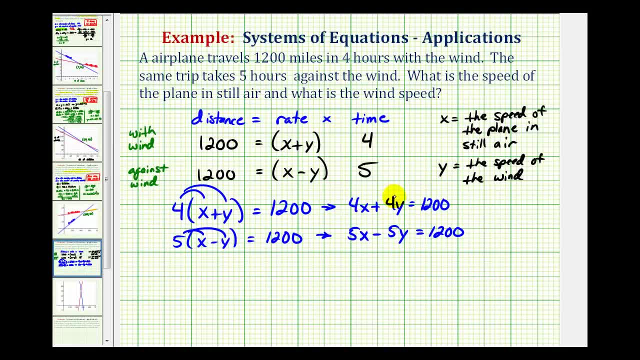 And since the least common multiple of four and five would be 20,, if this was plus 20y and this was minus 20y, the y terms would be eliminated When we add the two equations. So to do this, we're going to multiply this first equation by positive 5,. 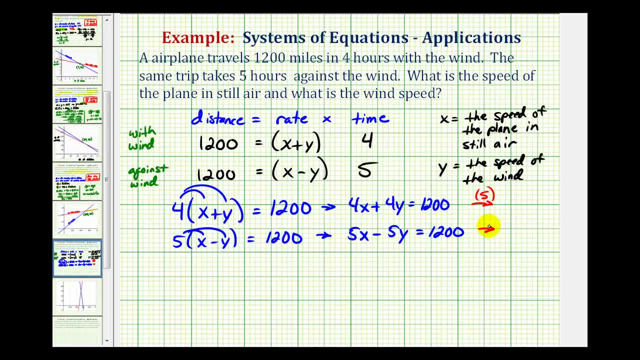 giving us a positive 20y here, And multiply the second equation by positive 4. This would give us a negative 20y here. So multiplying the first equation by 5 would give us 20x plus 20y equals 1,200 times 5 would be 6,000.. 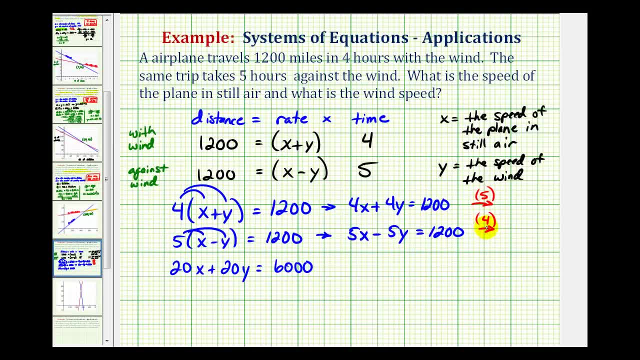 Now we'll multiply the second equation by 4.. So we're going to have 20x minus 20y equals 1,200 times 4 would be 4,800.. And now notice: when we add these two equations together, the y terms are opposite. 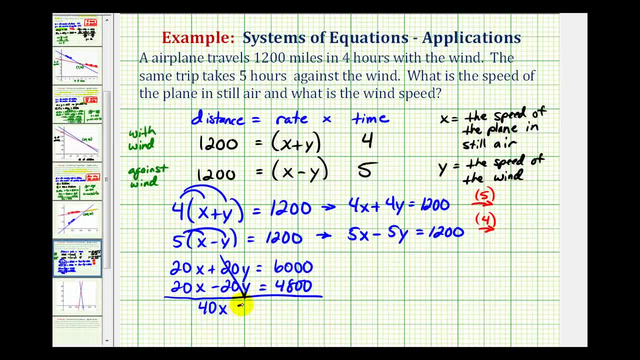 So this would be zero. So we have 40x equals. this would be 10,800.. So we'll divide both sides by 40.. This would be x, And 10,800 divided by 40 is equal to 270.. 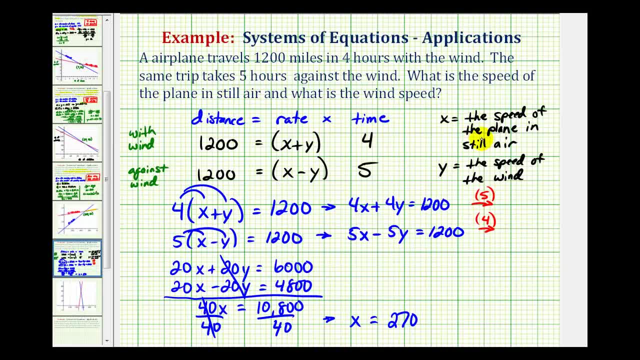 So now we know the speed of the plane in still air is 270 miles per hour, But we still have to determine the speed of the wind. So let's go ahead and use this equation here: Substitute 270 for x and then solve for y. 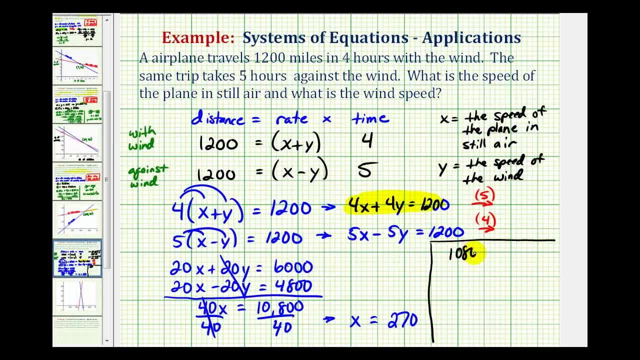 Well, 4 times 270 is 1,080, plus 4y Must equal 1,200.. Subtract 1,080 on both sides Should be zero. So we have 4y equals. this would be 120.. 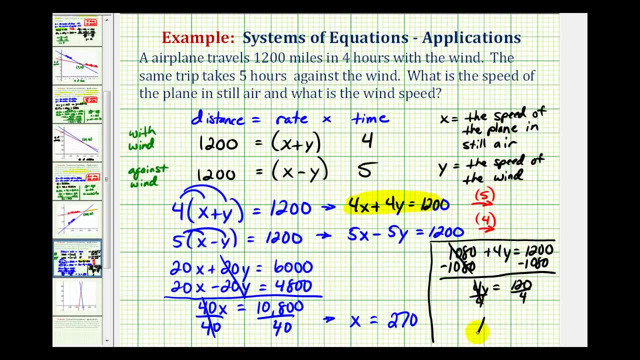 Divide both sides by 4.. So we have: y equals 120. divided by 4 is equal to 30.. So to answer the question, what is the speed of the plane in still air and what is the speed of the wind? the plane?